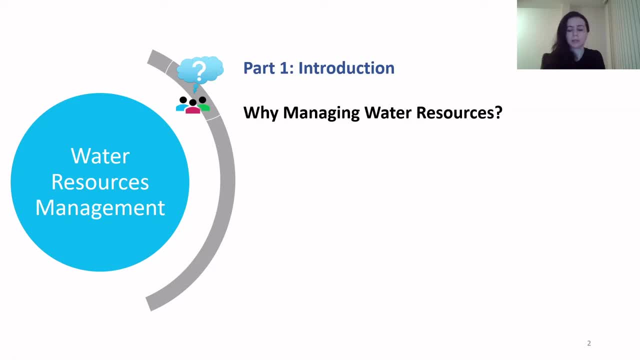 do it and what are the consequences of managing water resources? In the second part, we're going to talk about simulation and modeling of the water resources systems and how we can use this simulation tool to help us better manage our water resources. Finally, we are going to have 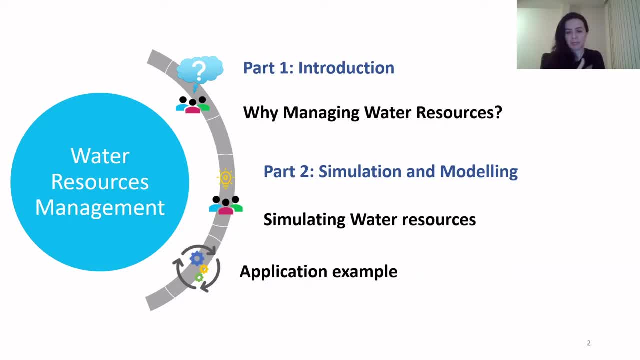 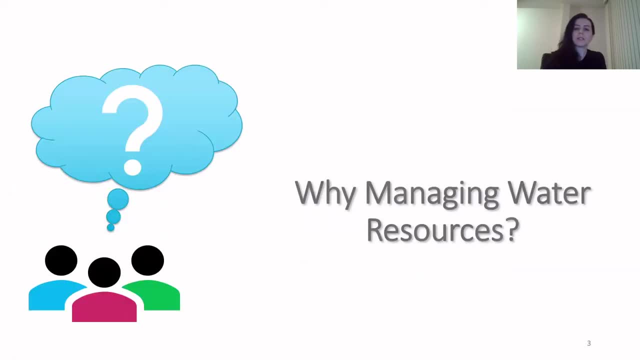 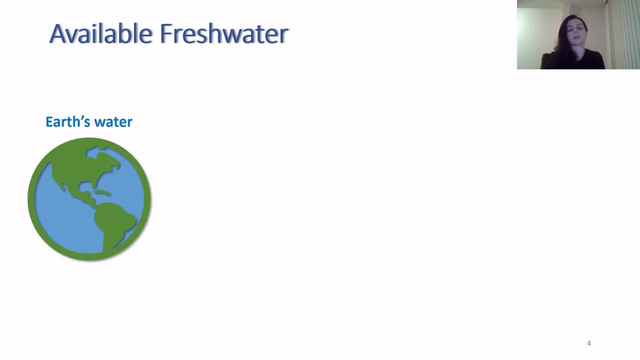 a look at an application example to showcase the application of these simulating water resources models. Let's start with finding out why we need to manage our water resources. When we look at Earth, we can see water everywhere, So why we need to manage water? Well, the fact is that from 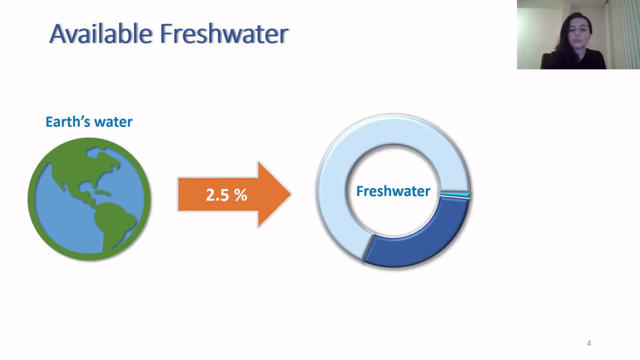 all water that we can see, only 2.5% is fresh water, meaning that the rest is salt water and not suitable for human usages like drinking or irrigating crops. Even from this 2.5% of fresh water that we see here, the rest is Beachy- yeah, in the form of glaciers and ice caps, not 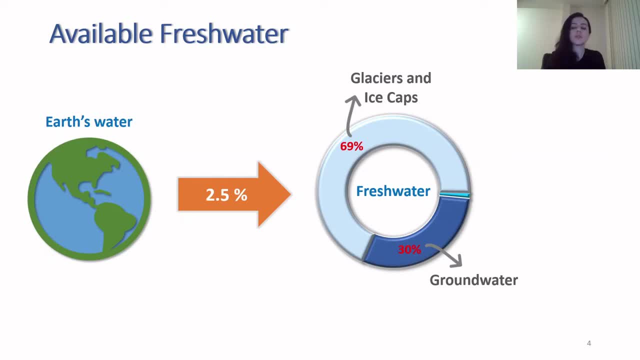 easily accessible. 30% of this fresh water is in the form of groundwater: easier to access but expensive because we need to use pumping facilities and electricity to extract water from the deeper layers on the ground. Only 1% of this fresh water. much has been covered by wet. 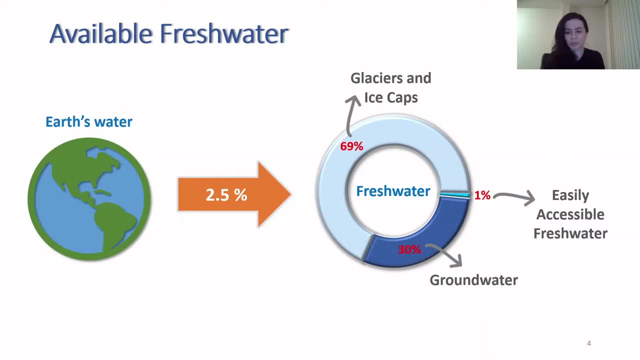 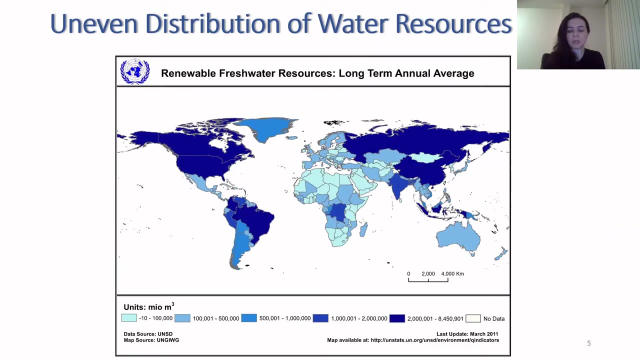 monday in the call. water in the form of the from them helpingጌht. second part is in the is considered as easily accessible fresh water, and that is the water that mostly is available through rivers and lakes. Another reason that we need to manage our water resources is that this limited amount of water is not distributed. 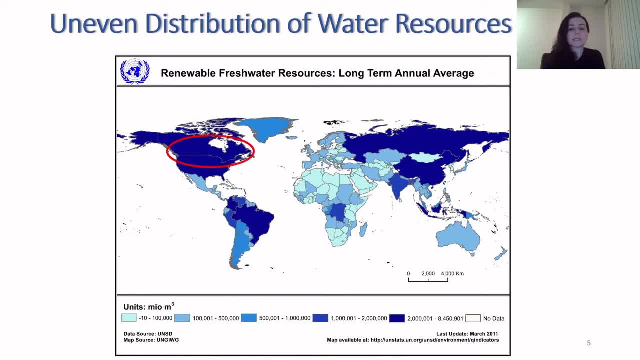 across the world evenly. There are countries like Canada where water is abundant, versus countries like North African countries with very limited access to fresh water. Even in many parts of the world, temporal distribution of water resources and the availability of fresh water is not considered evenly. So in these parts, like many semi-arid or arid areas, 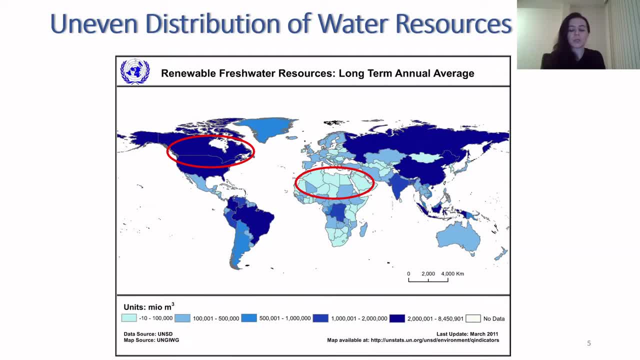 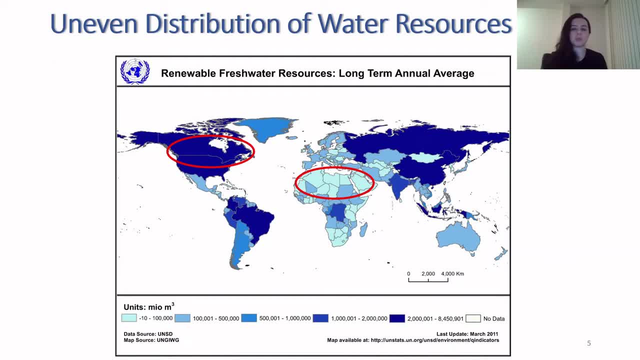 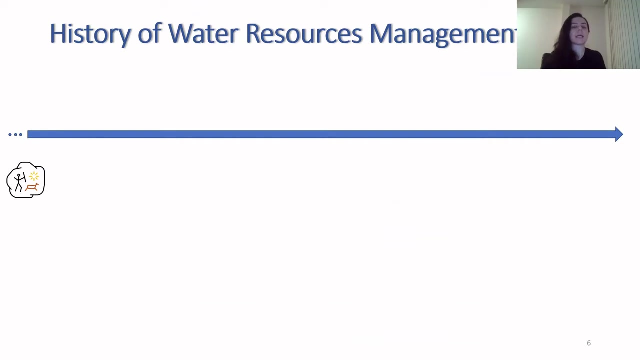 So we see that the distribution of fresh water and its availability does not match our requirements. That's why we need to manage water resources to actually match the distribution and availability of fresh water to our demands for fresh water. Fresh water resources and water resources management is not something new to humans. 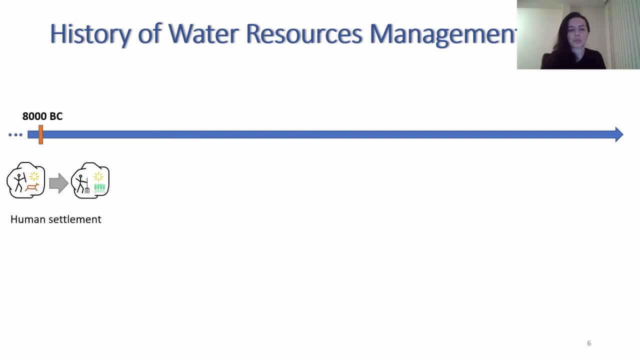 Actually, humans started managing water resources when they started settling down Around the sources of water to practice agriculture. instead of hunting and gathering, Those days, humans tried to make their homes and their farms as close as possible to the sources of water to be able to grow their own foods. 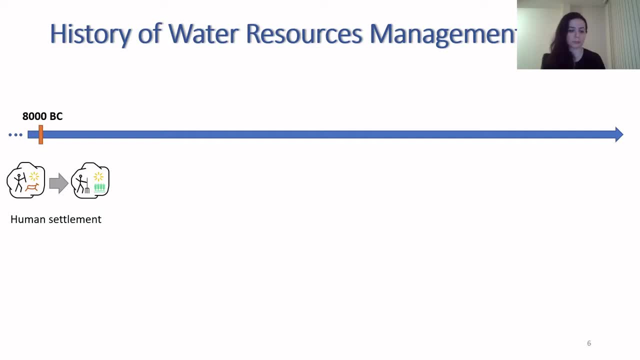 But by growing a population. it was not that easy to find springs But close to the source of water to make a farm or a house. Also, sometimes because of flooding events and some other natural disasters it was even dangerous to live that close to rivers and other some other sources of water. 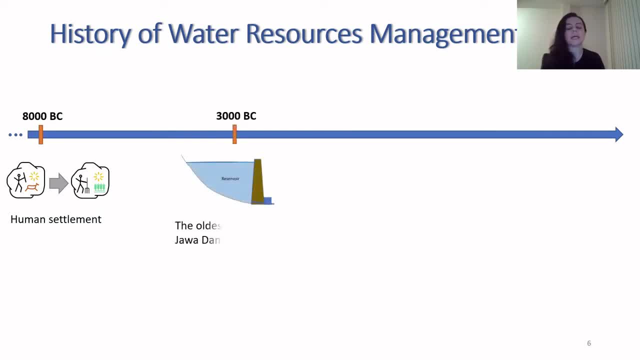 So humans started to learn how to build dams and how to store water in reservoirs when it was abundant, To use water when it was needed. The oldest known dam dated back to almost 3000 BC. Since those days, humans continue to to grow their communities and started to form cities and practice urbanized life lives. 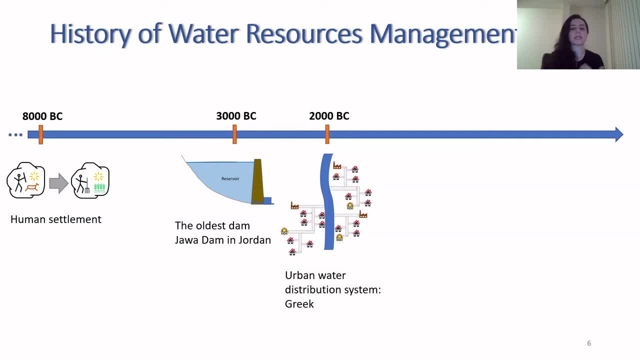 In those days, humans constructed and constructed urban water distribution systems and sewer systems for their ancient cities. One of the examples have been found in ancient Greek cities around dated back to around 2000 BC, And it was around those years that people started transferring water from where it originates. 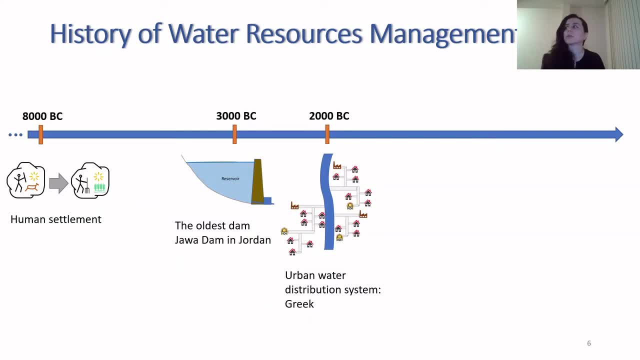 To where it can be used. So some examples include Roman aqua ducts, the elevated aqua ducts, the elevated ducts, or pathways to transfer water from mountains to Roman cities, And or some other underground pathways to convey water invented by people in ancient Persia called Kanat. 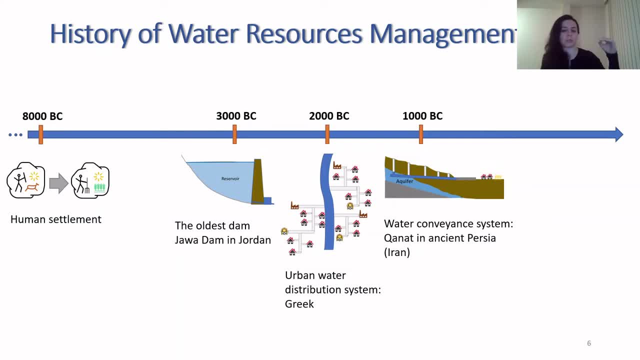 Which was designed to transfer water from from mountainous aquifers to the plains where people lived. Also, people learned how to divert water from rivers, to use it and to irrigate their farms, and how to control flood. So one of the oldest irrigation and flood control systems is found in China, around 256 years ago. 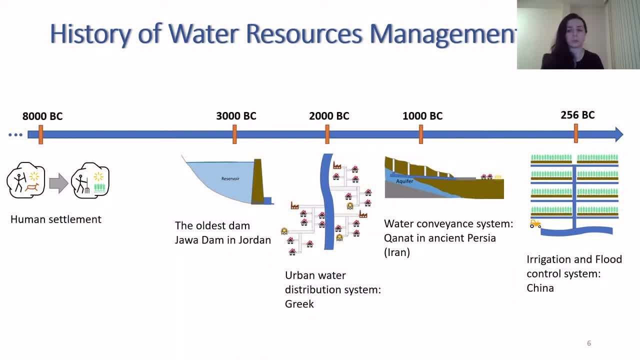 So one of the oldest irrigation and flood control systems is found in China around 256 years ago. So one of the oldest irrigation and flood control systems is found in China around 256 years ago And it's still working nowadays. So you can see that the history. 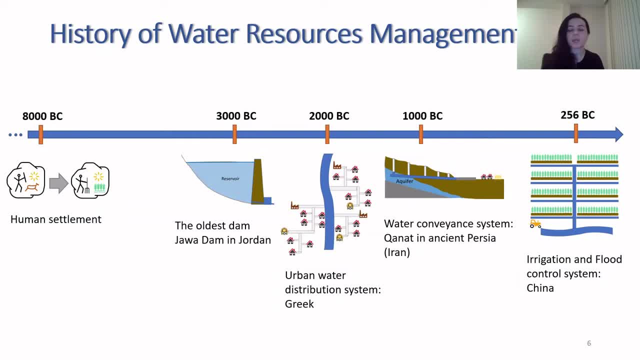 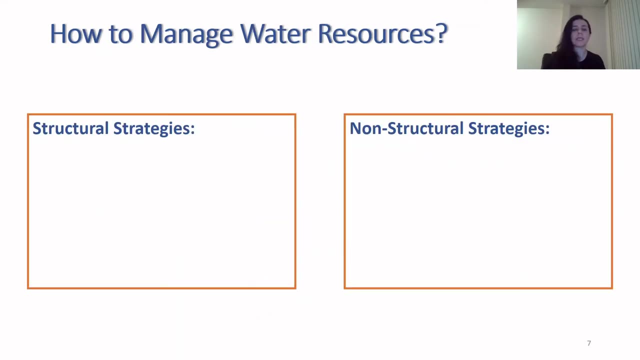 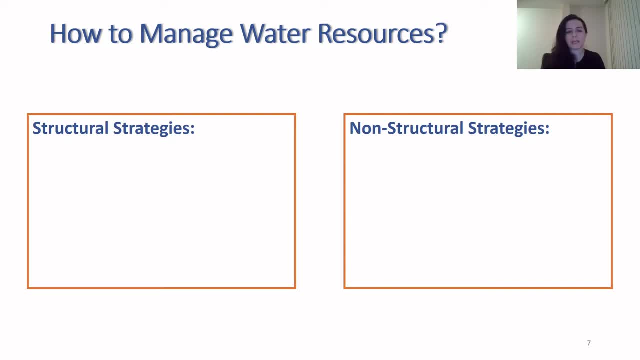 Now, if we want to categorize water management strategies, we can consider two main categories: structural and non-structural strategies. an example of structural strategies is reservoir construction. so we build a dam to form a reservoir and to store water when it's abundant and use it when we need it. also, we can transfer water. 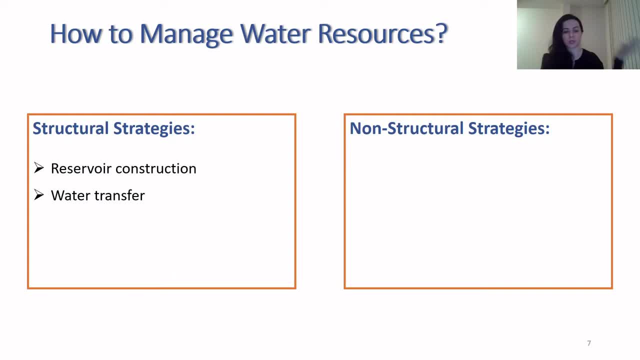 from, let's say, mountains, when it is originated, to cities where we need to use it. there are other structural strategies, like recycling or treatment of used or pollutant water, and that used to be mainly the case for industries that do not need high quality fresh water for their production. 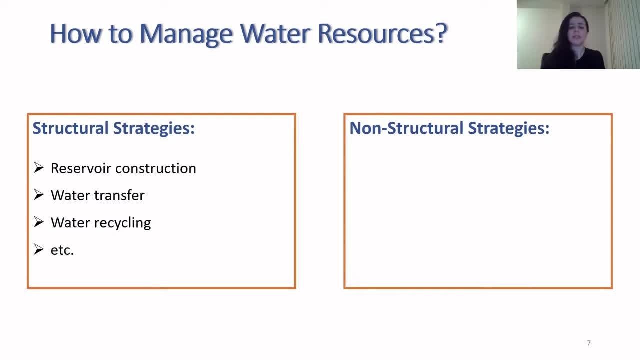 but nowadays, researchers are finding and working on methods to recycle and to treat pollutant water to the degree that is suitable even for drinking purposes. non-structural strategies, on the other hand, are mainly focused on managing water demand or water allocation. how can we manage water demand? 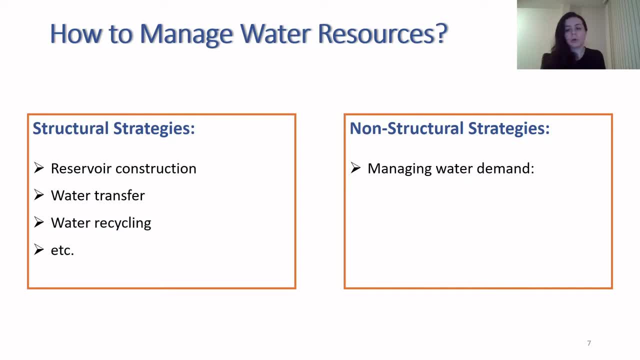 well, take a farm as an example. in a farm where crop types are highly water demanding, we have a high demand for water, but if we replace those crop types with with with some other types of crops that require less water, or even if we replace the crop hide highly water demanding crops with another, 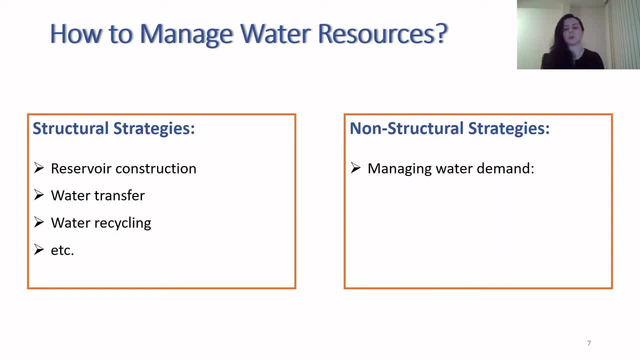 variety of the same type but with lower water demands, we can reduce the the total amount of water requirement for that farm. so you can see that this is one of the ways that we can manage our demand for water. also, we can manage the way that we allocate water. so if we reduce water, 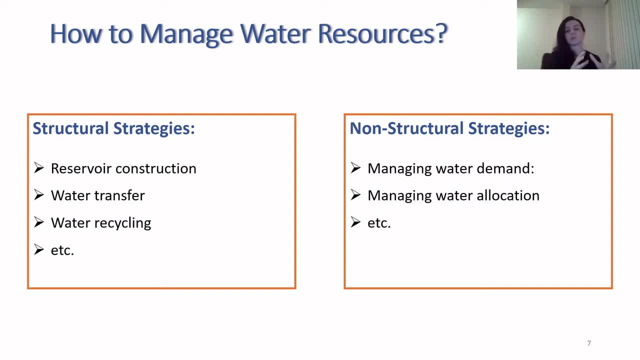 that is allocated to one sector and pass that water to another sector that can generate more economic benefit using the same amount of water. we are almost managing our water allocation. and there are so many other examples and, as you may have noticed this, these examples, under both categories, are mainly focused on quantitative management of 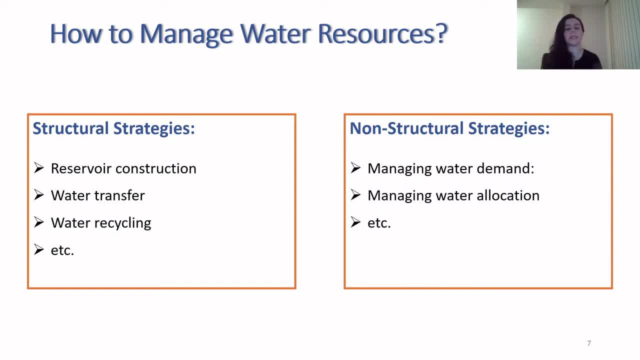 water resources, whereas there are so many other examples of other ways of managing water resources that are associated with water and are associated with other issues that we face, like flood control or water quality management. for the sake of time and to keep it simple, here i'm focusing on water. 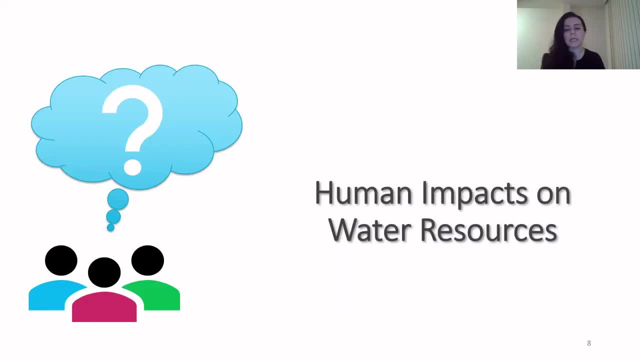 on quantitative management of water resources. when we manage our water resources, actually, we are to match the timing and the amount of available water to our requirements. Whatever change that we make to the natural system has some consequences, So let's see how we impact the water system when we try to manage these systems. 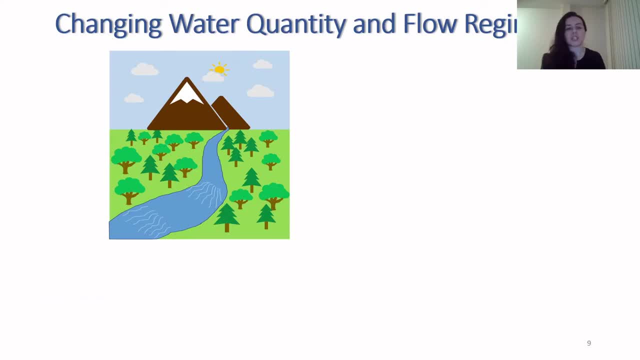 One major change that we usually make to the water systems is changing the quantity and the flow regime. Take a river before being changed by humans as an example. Perhaps this river has a monthly distribution, flow distribution like what you can see on the screen right now, shown in a black dotted line. 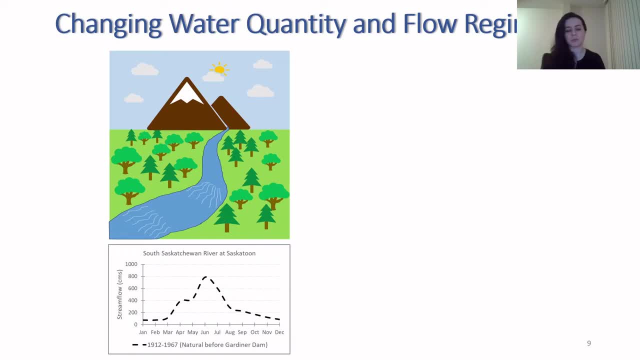 This graph is based on observed data for the South Saskatchewan River at Saskatoon, here in Canada, the city that I'm living in now. Now imagine that humans find this river and they like it and they want to settle down around this river. So they start to make their homes, start to practice agriculture, cultivate their crops. 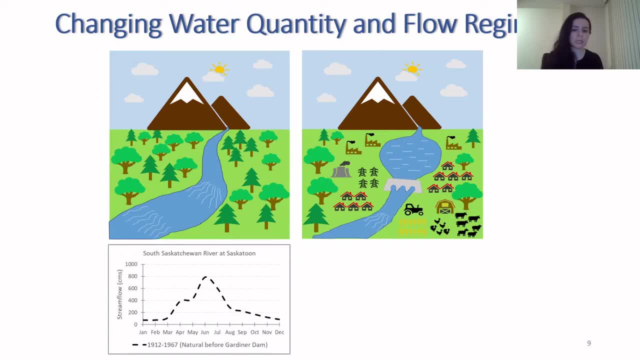 and raise their livestock and also they establish their factories all around the river. To supply water to all these demands and all these different users, they need to build a dam on the river to store water. So this is the reservoir behind the dam. 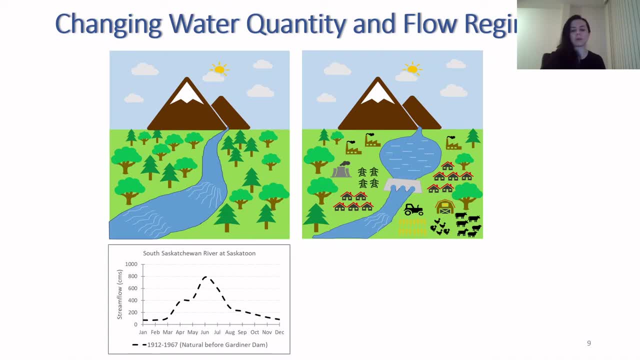 And now, if you look at the monthly distribution of this river- the same river, but after the construction of the dam- you can see that the quantity and flow regime changes dramatically. So the peak flow that used to occur around June at the level of almost 800 cubic meters per second. 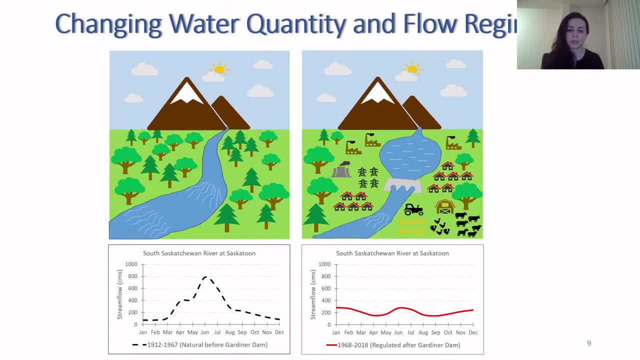 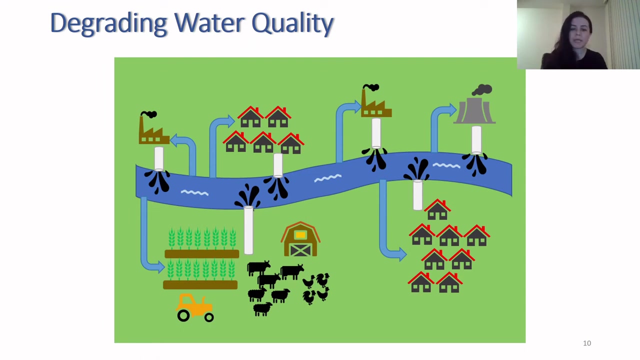 now dropped down to almost 300 cubic meters per second. So this is one way that we impact the natural system when we try to manage water resources. Also, apart from this quantitative impact, we may degrade the quality of water resources, And a very simple example of that is when we extract water from rivers. 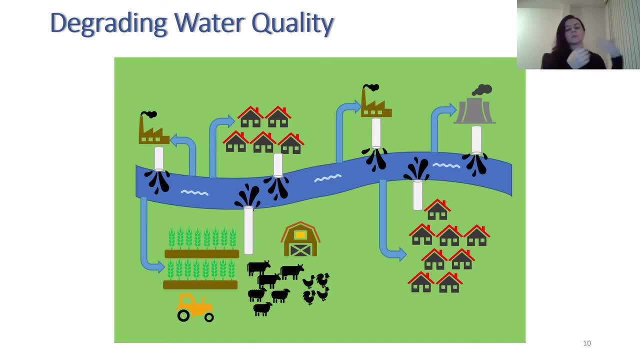 we can degrade the quality of water resources, And a very simple example of that is when we extract water from rivers. we can degrade the quality of water resources, So we can extract water from the river, for example, and then use it to irrigate our lands. 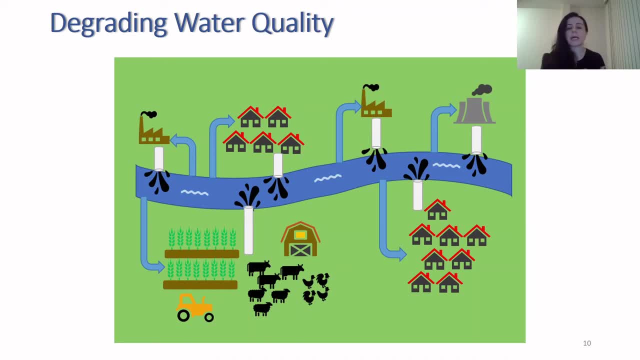 and at the same time use fertilizers and pesticides- in general, chemicals- which is mixed with the water, and then return that pollutant water to the river. So we are degrading the quality of the river by discharging these pollutants. So we are degrading the quality of the river by discharging these pollutants. 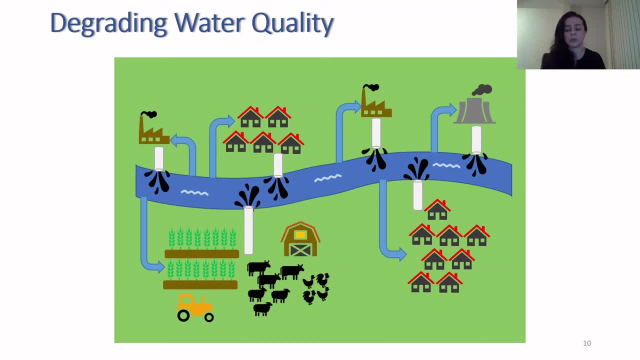 efflores into the river. So this is dangerous in the sense that we might reach to the point where the water in this river is not suitable for human usages. So this is dangerous in the sense that we might reach to the point where the water in this river is not suitable for human usages. 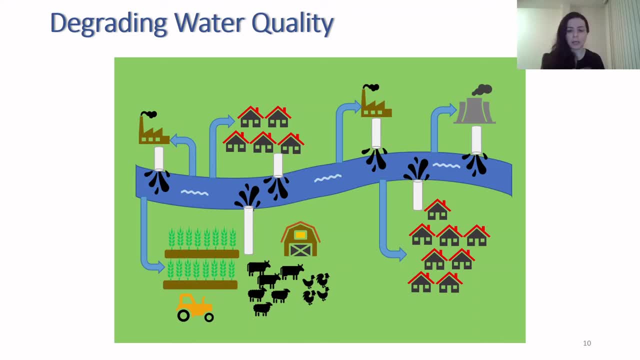 like drinking or irrigation anymore because of the high level of contaminants in it. So, as discussed, our different water management strategies have consequences on the environment and on other users. So, as discussed, our different water management strategies have consequences on the environment and on other users. 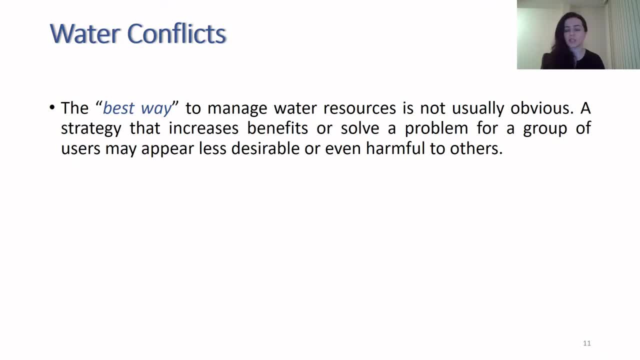 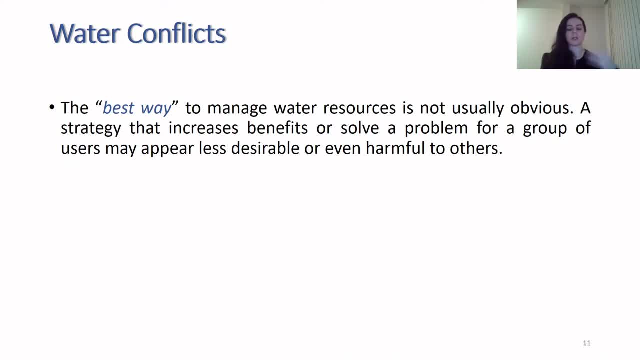 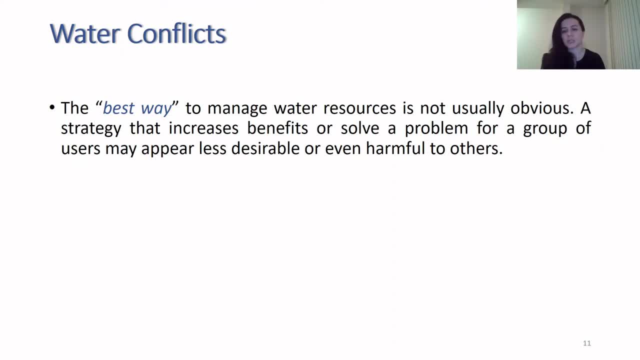 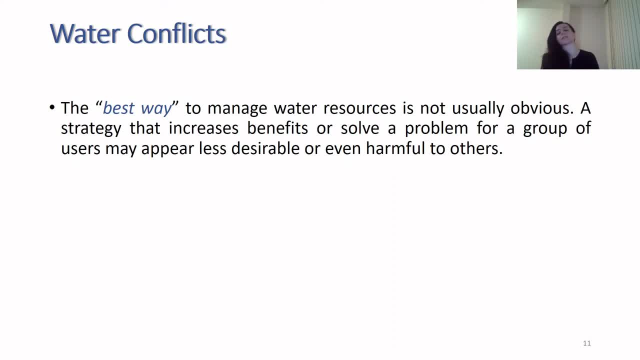 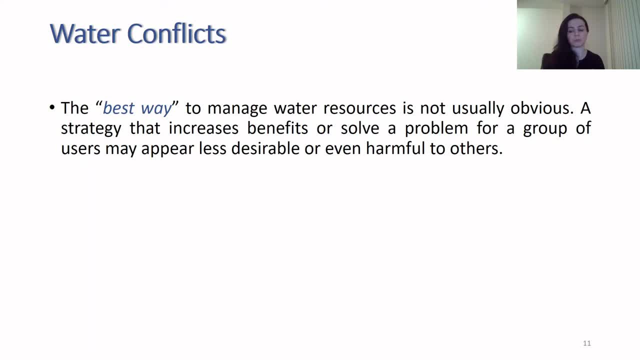 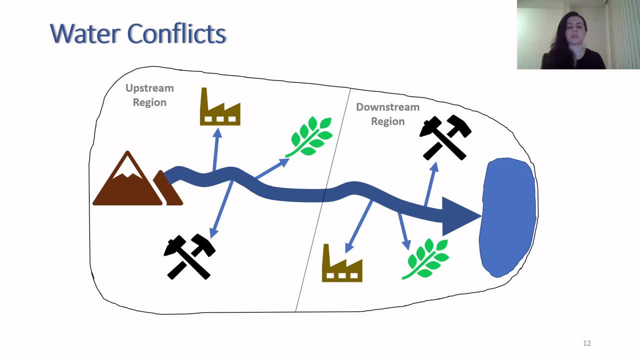 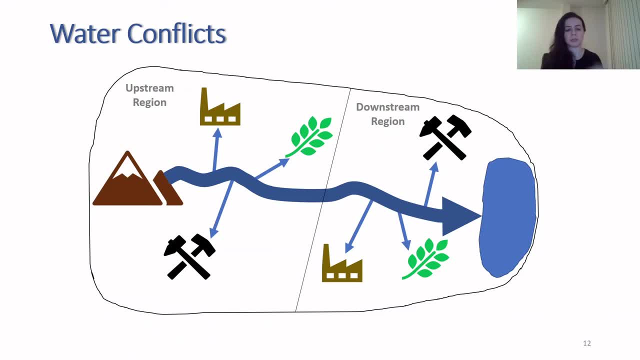 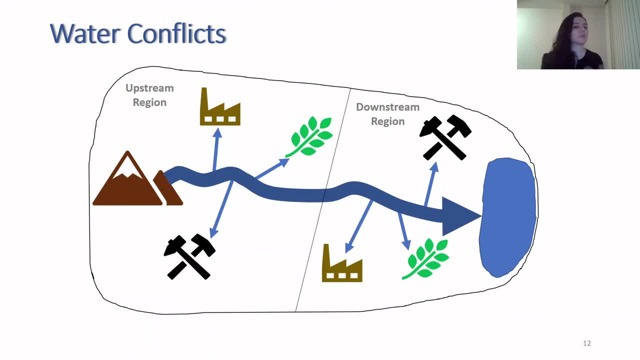 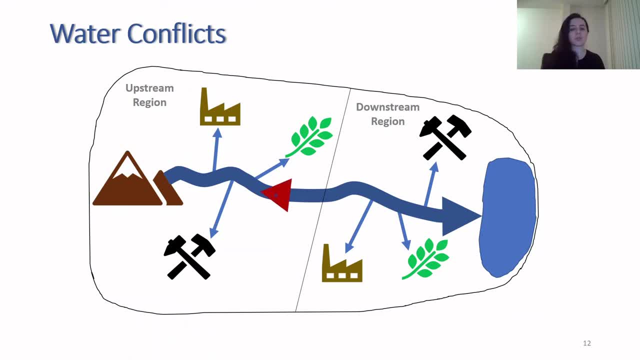 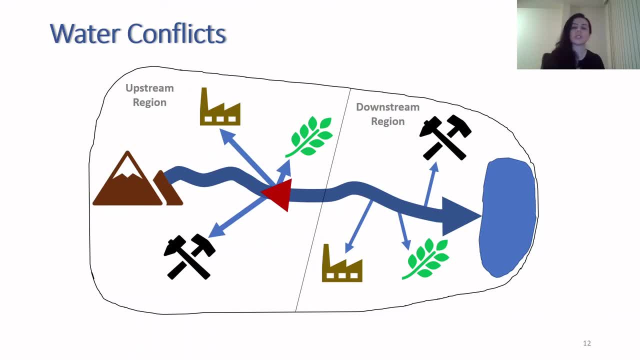 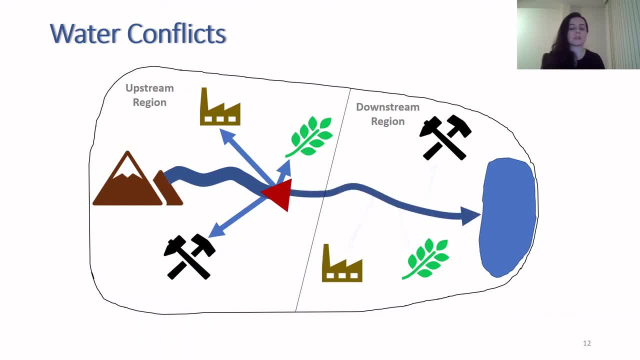 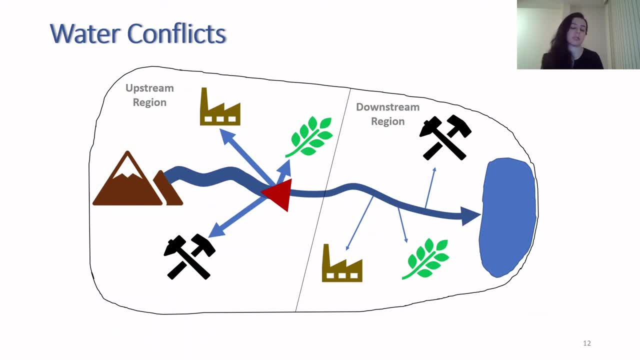 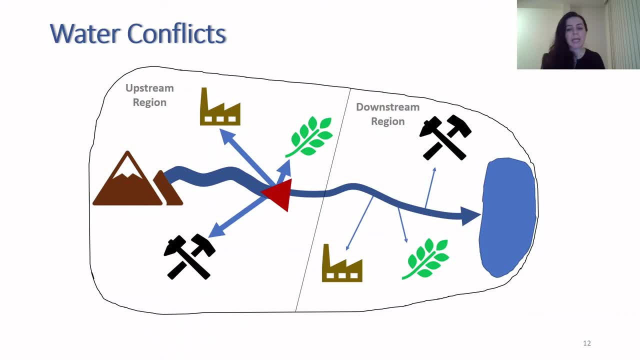 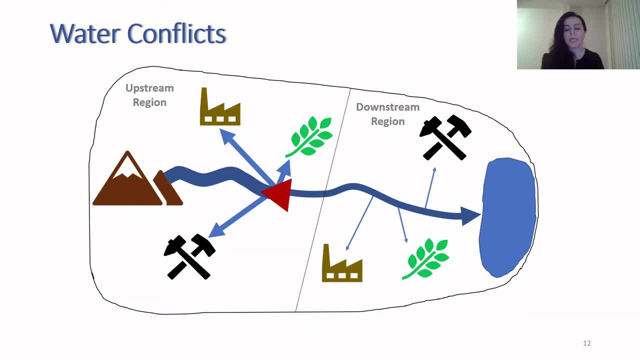 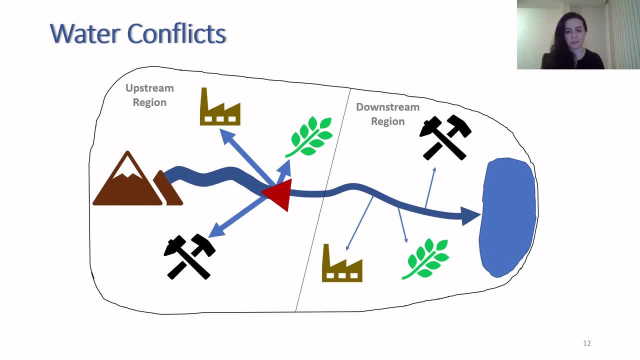 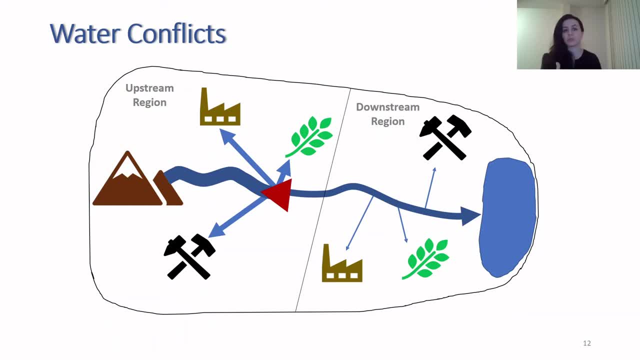 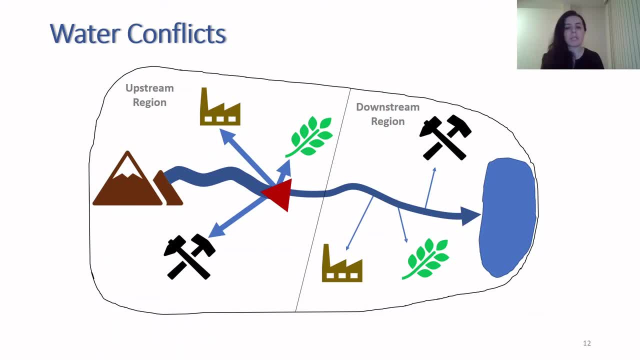 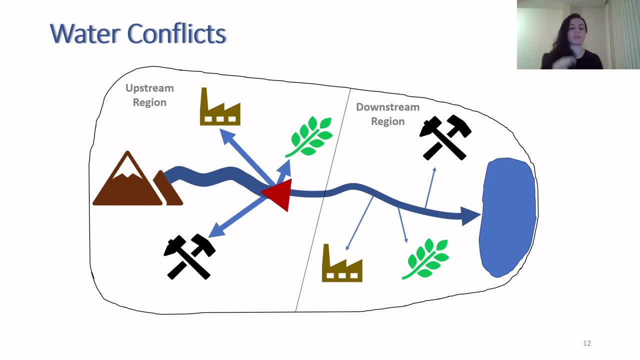 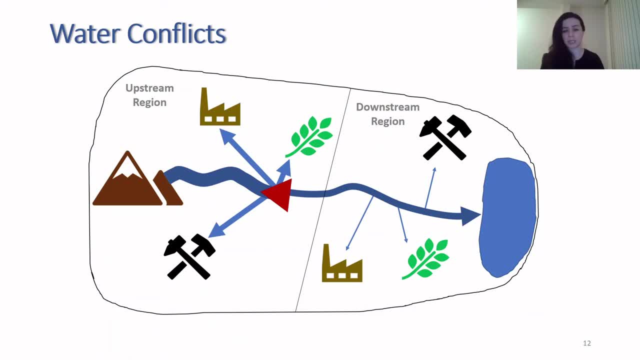 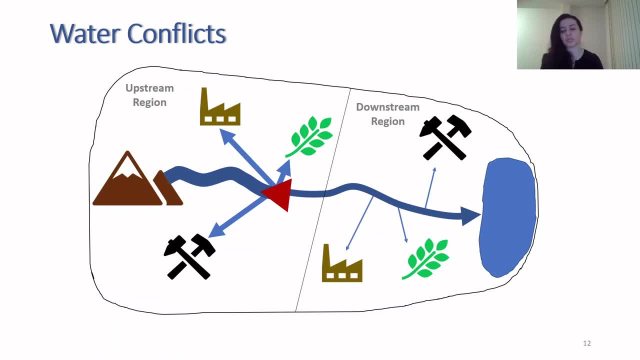 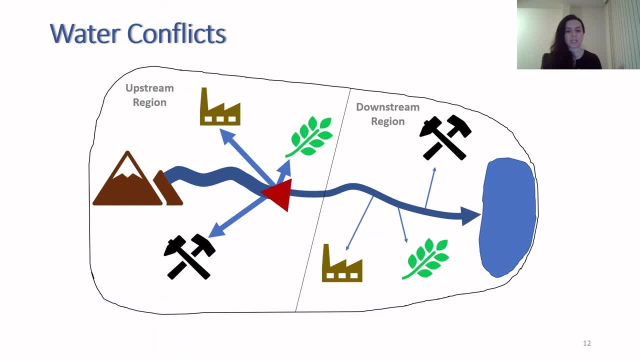 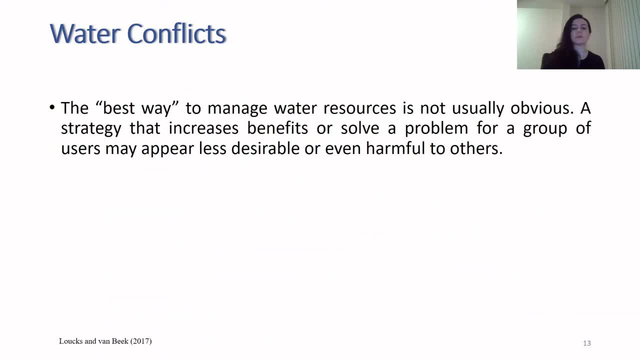 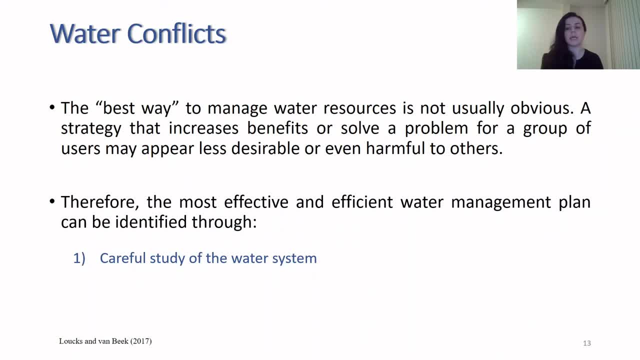 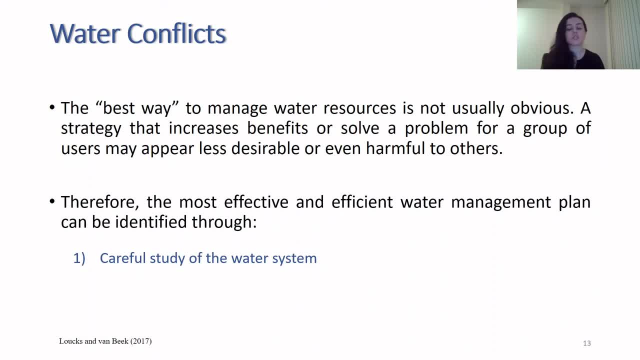 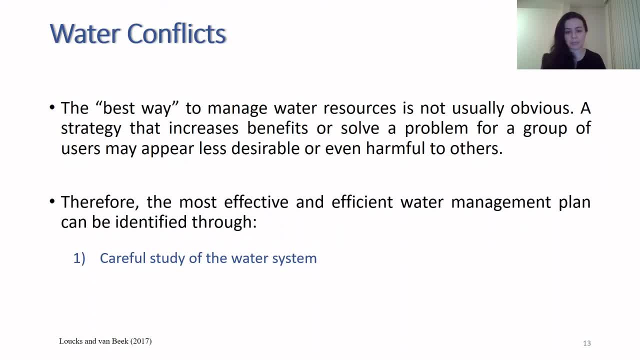 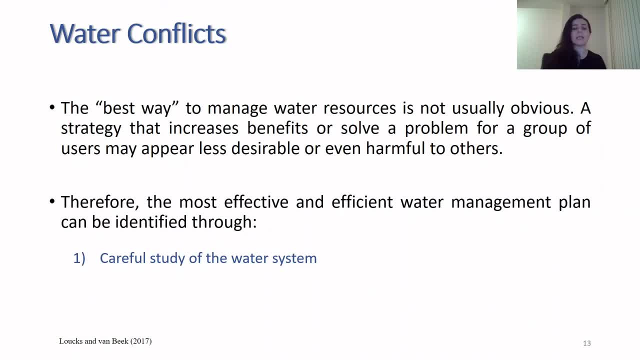 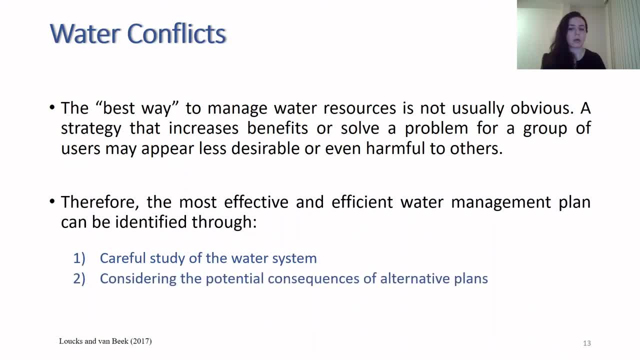 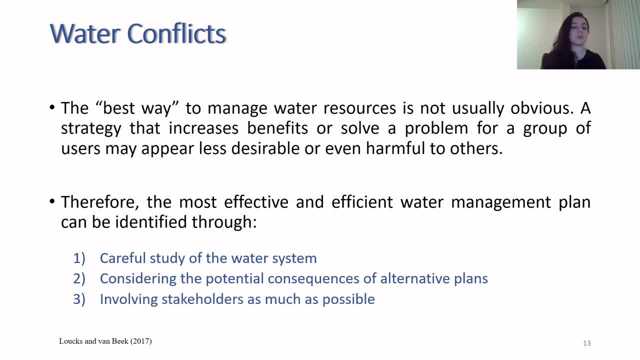 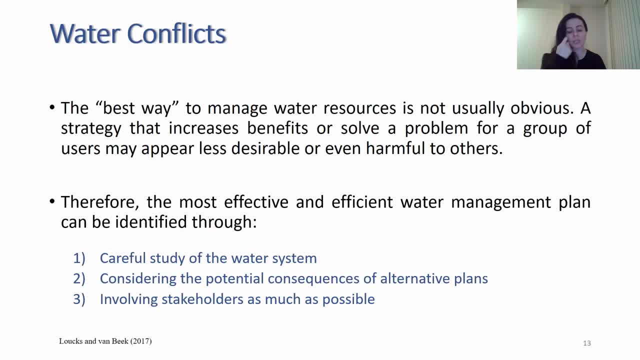 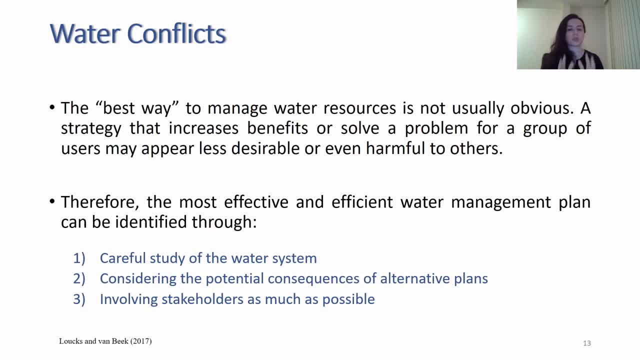 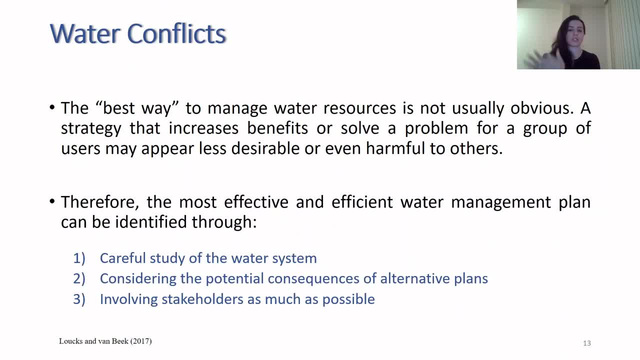 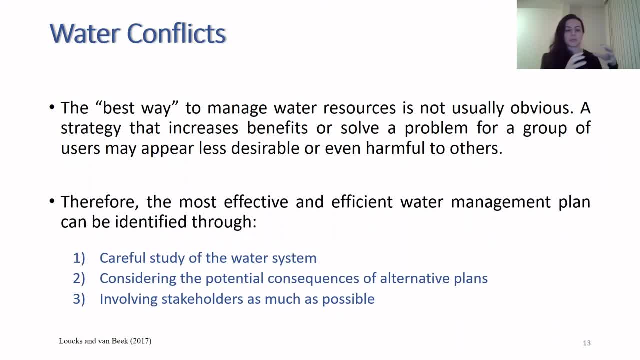 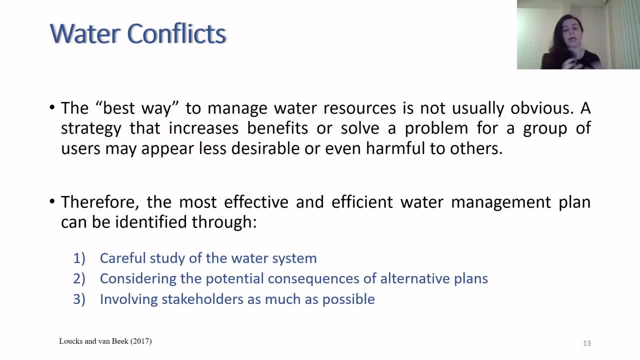 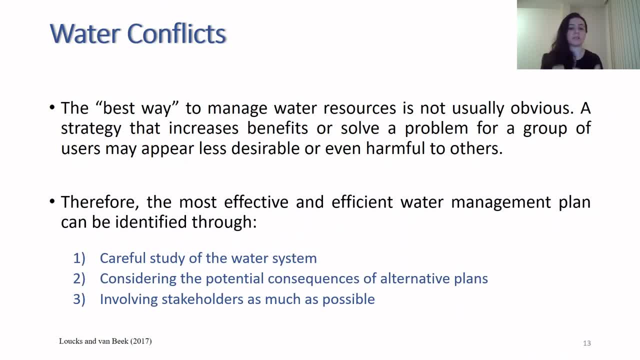 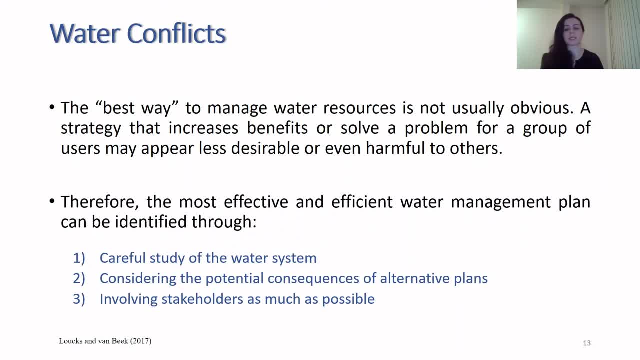 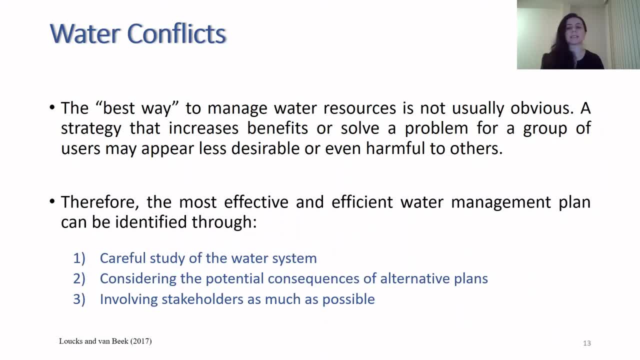 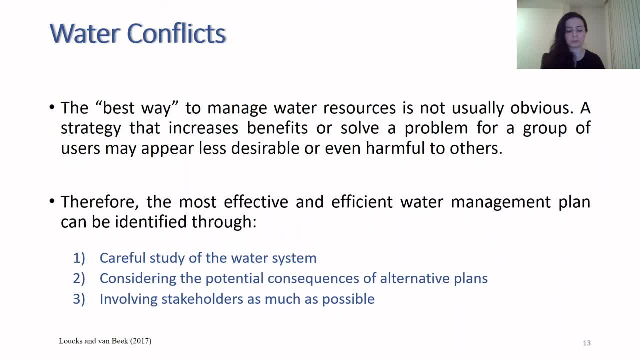